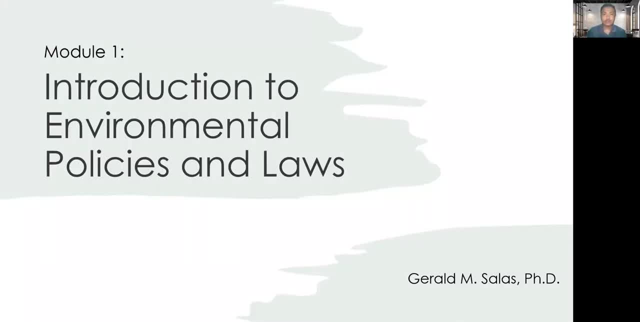 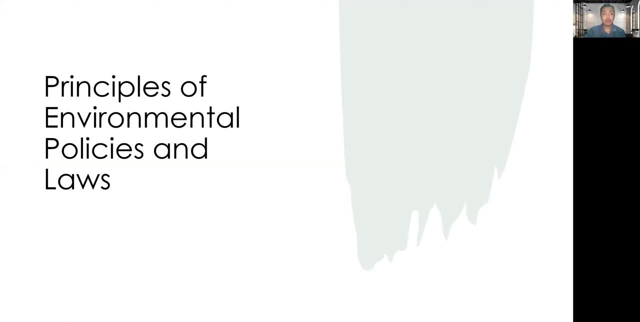 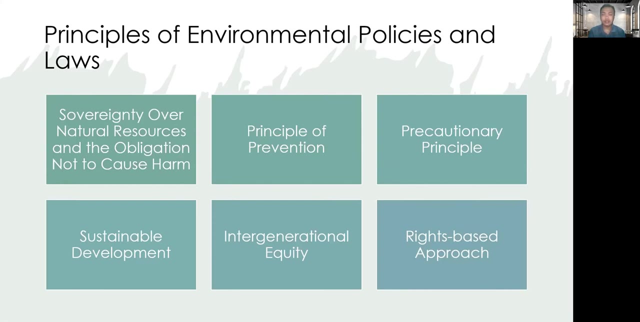 This is Module 1, Introduction to Environmental Policies and Laws. To start our discussion, we'll talk about first the principles of environmental policies and laws. There are various principles in which environmental policies and laws are anchored. First, sovereignty over natural resources and the obligation not to cause harm. 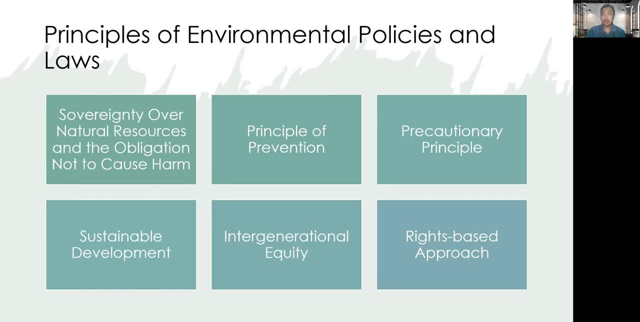 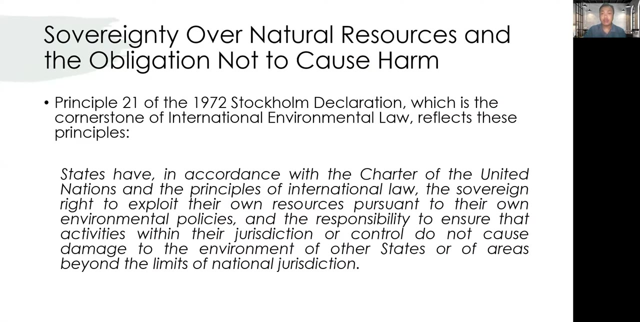 Second, principle of prevention. Third, precautionary principle. Fourth, sustainable development. Fifth, intergenerational equity. And sixth, the rights-based approach. The Principle 21 of the 1972 Stockholm Declaration, which is the cornerstone of international environmental law, reflects these principles. 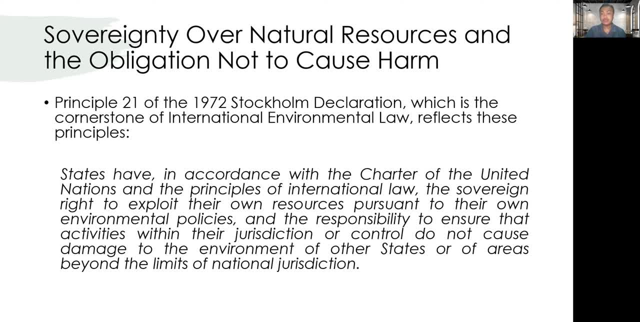 States have, in accordance with the Charter of the United Nations and the principles of international law, the sovereign right to exploit their own resources pursuant to their own environmental policies and the responsibility to ensure that activities within their jurisdiction or control do not cause damage to the environment of other states. 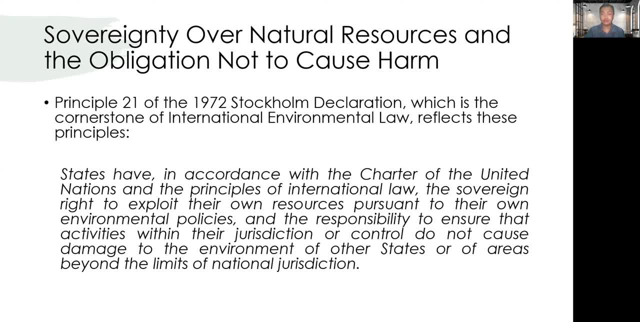 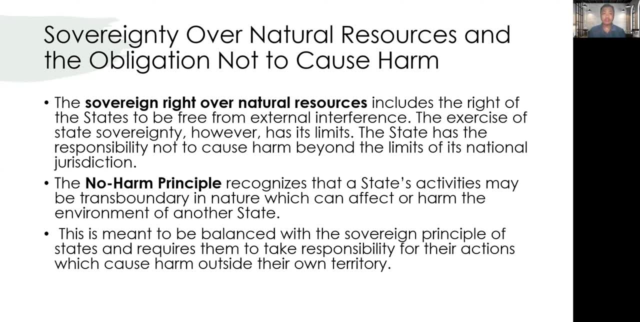 or of areas beyond the limits of national jurisdiction, Meaning the sovereign right over natural resources includes the right of the states to be free from external interference. The exercise of state sovereignty, however, has its limits. The state has the responsibility not to cause harm beyond the limits of its national jurisdiction. 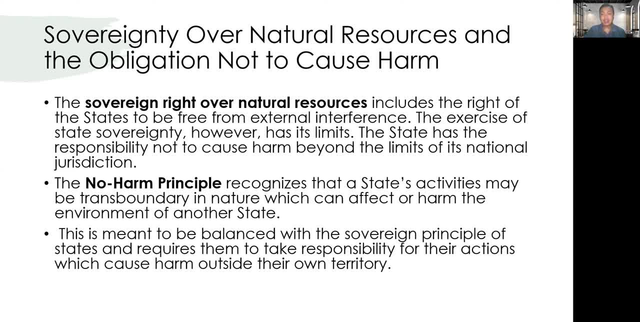 The no-harm principle recognizes that a state's activities may be transboundary in nature, which can affect or harm the environment of another state. This is meant to be balanced with the sovereign principle of states and requires them to take responsibility for their actions which cause harm outside their own jurisdiction. 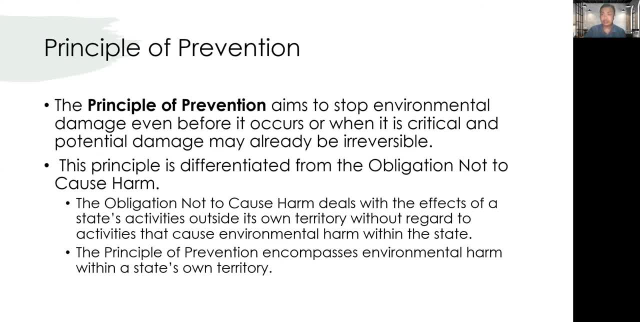 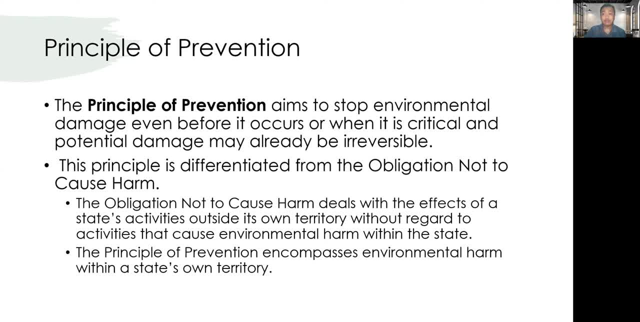 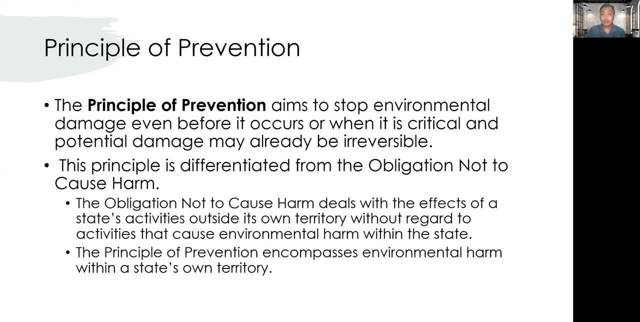 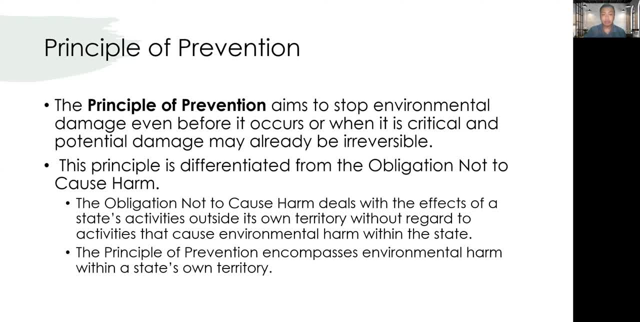 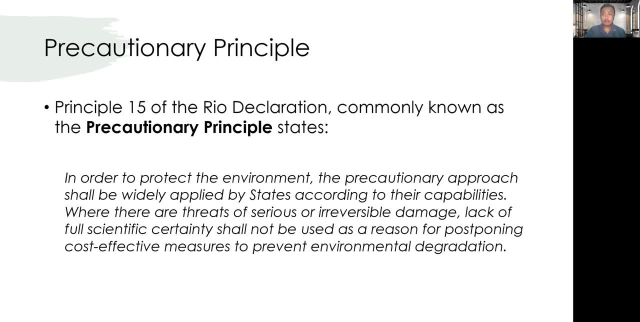 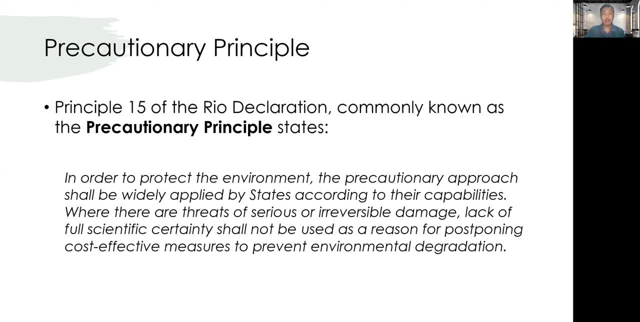 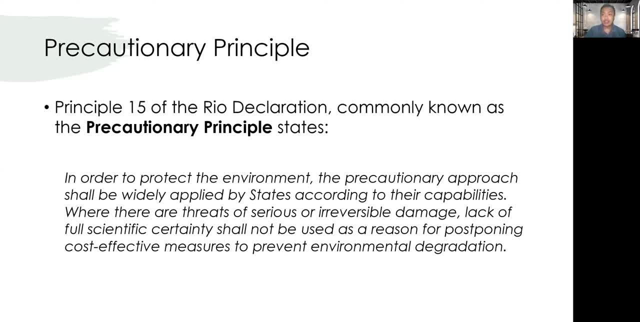 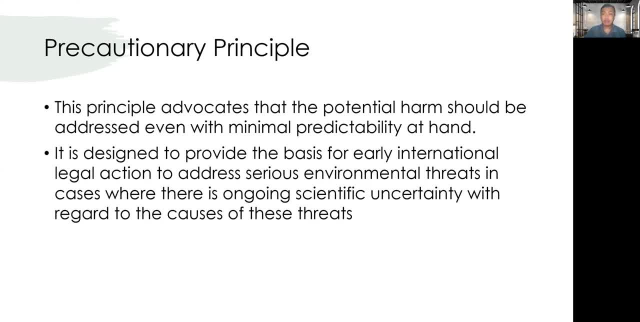 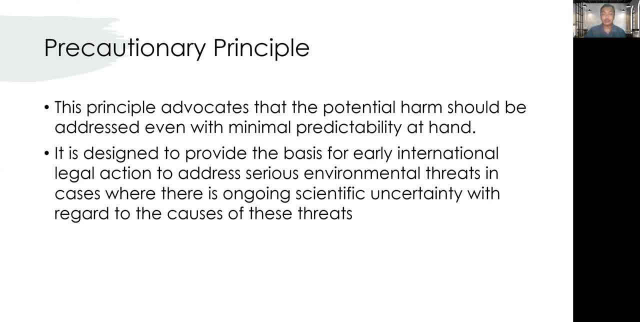 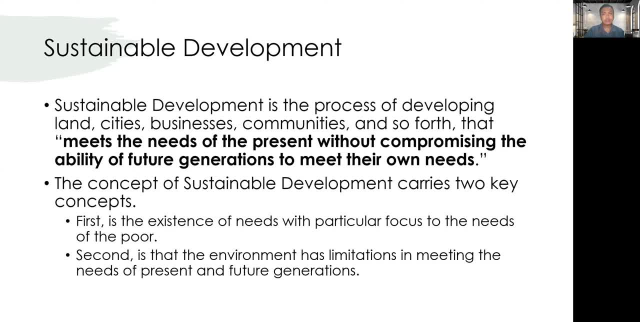 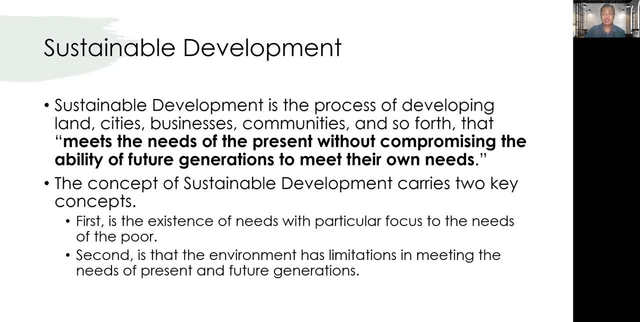 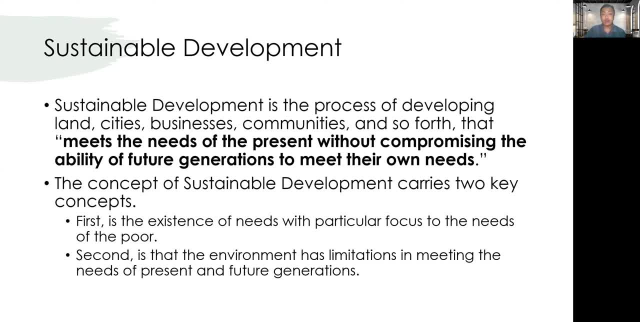 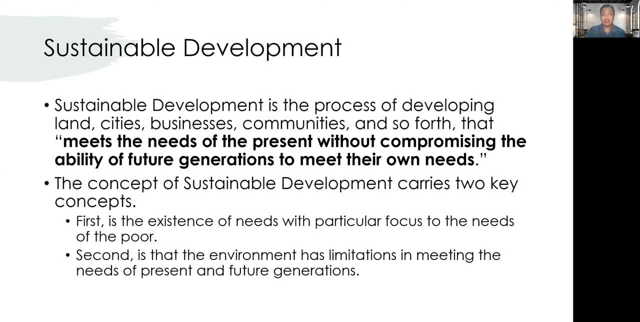 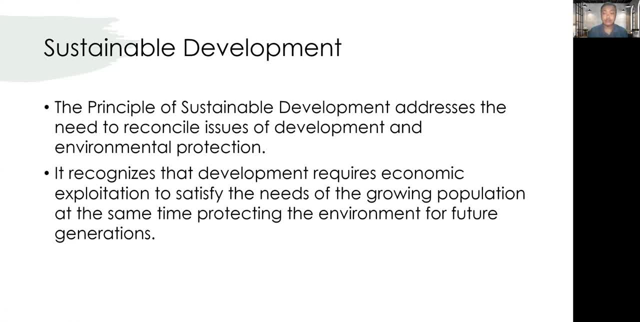 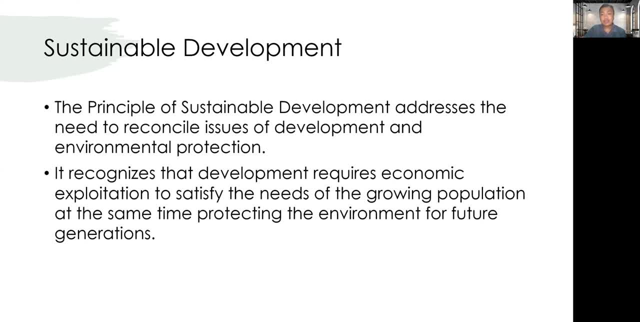 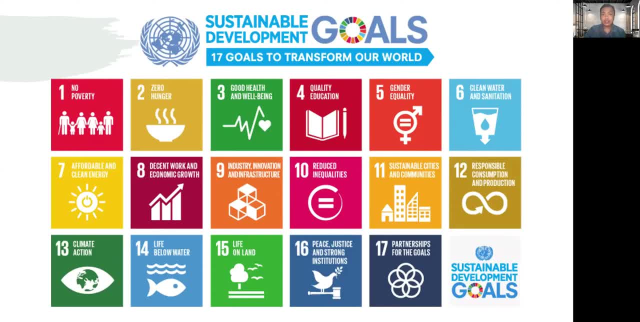 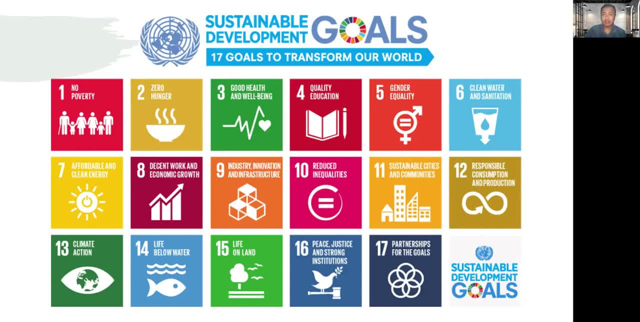 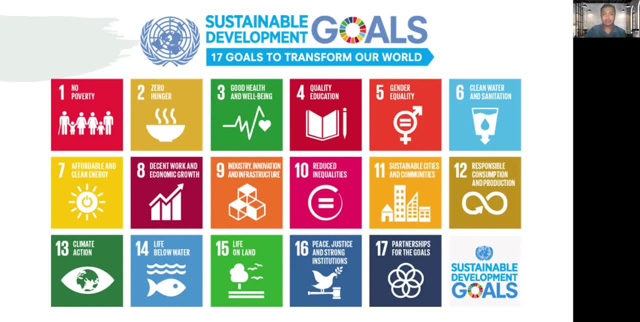 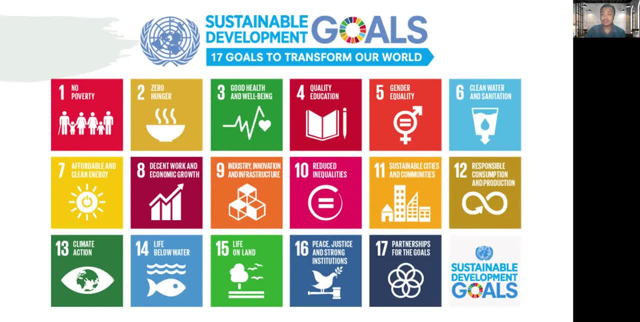 which can affect or harm the environment of another state. sustainable cities and communities. 12, responsible consumption and production. 13,. climate action. 14, life below water. 15, life on land. 16, peace, justice and strong institutions. 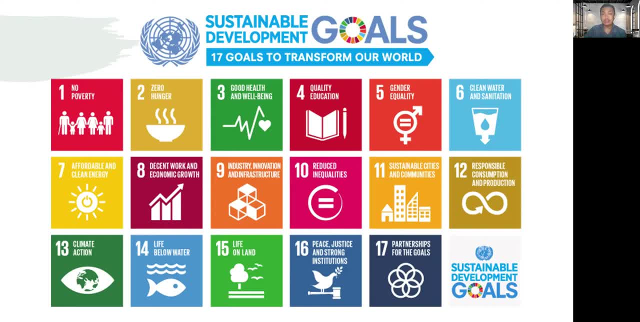 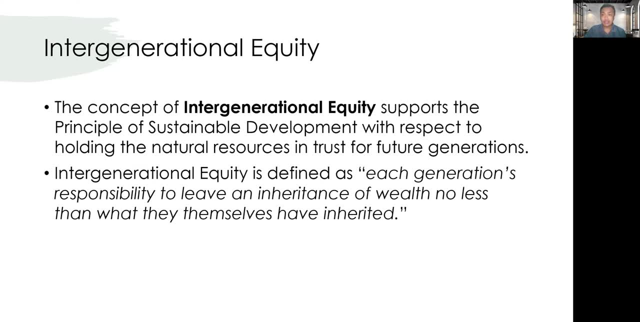 17, partnerships for the goals. These are the sustainable development goals. The concept of intergenerational equity supports the principle of sustainable development with respect to holding the natural resources in trust for future generations. Intergenerational equity is defined as each generation's responsibility to live an inheritance of wealth. 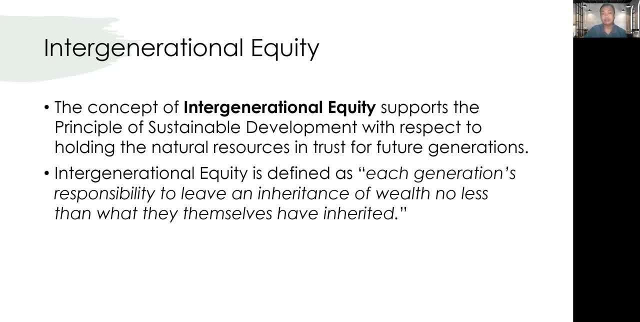 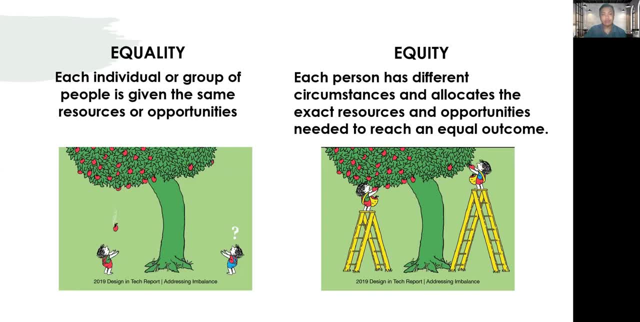 no less than what they themselves have inherited. These two images show you the comparison between equality and equity. In equality, each individual or group of people is given the same resources or opportunities. Meanwhile, for equity, each person has different circumstances and allocates the exact resources and opportunities needed to reach an equal outcome. 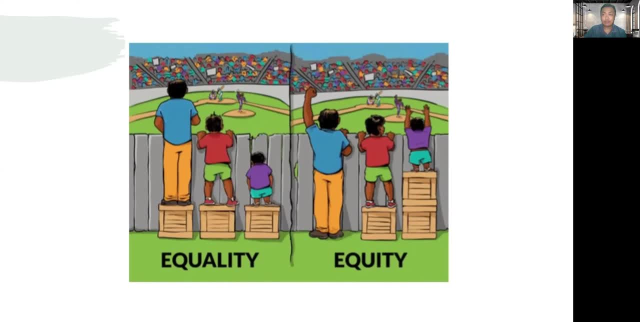 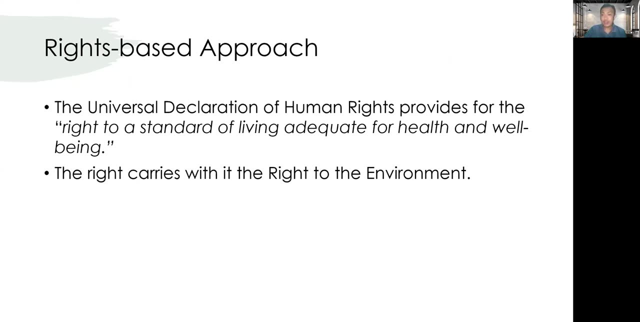 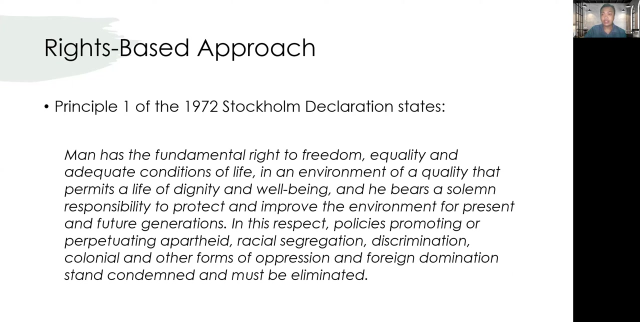 This image also shows you the comparison between equality and equity. The Universal Declaration of Human Rights provides for the right to a standard of living adequate for health and well-being. The right carries with it the right to the environment. In Principle 1 of the 1972 Stockholm Declaration states: 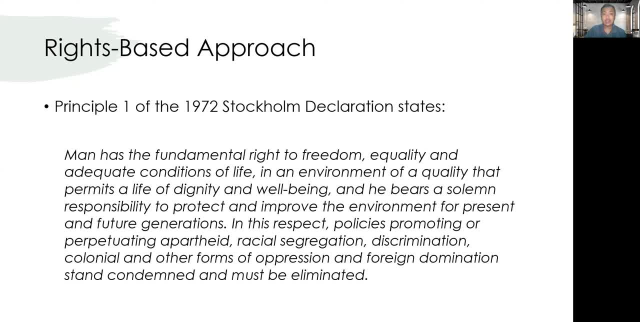 Man has the fundamental right to freedom, equality and adequate conditions of life in an environment of equality that permits a life of dignity and well-being, and he bears a solemn responsibility to protect and improve the environment for present and future generations. In this respect, policies promoting or preserving the economic security of the environment. 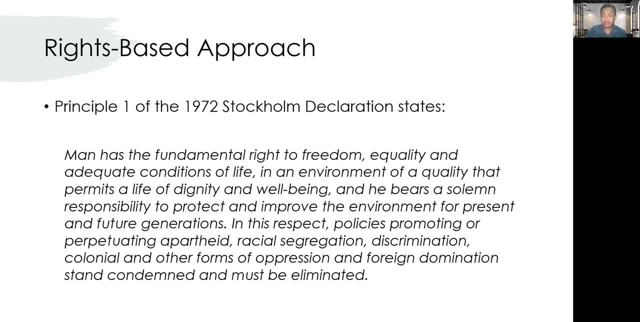 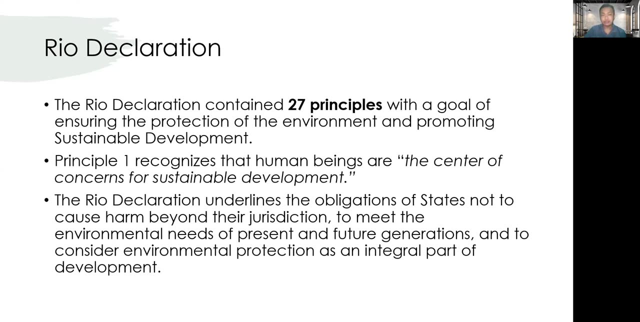 perpetuating apartheid, racial segregation, discrimination, colonial and other forms of oppression and foreign domination stand condemned and must be eliminated. This principle is further recognized by the Rio Declaration. The Rio Declaration contained 27 principles with the goal of ensuring the protection of the environment and promoting sustainable development In the 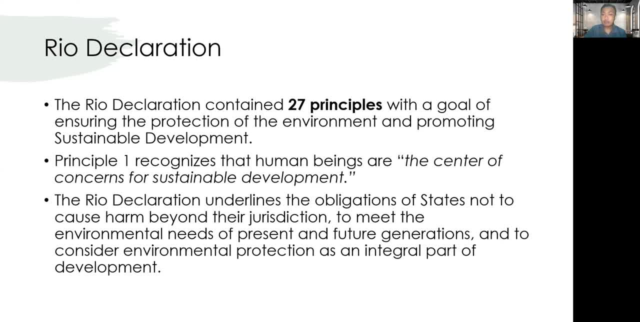 Principle 1 of the Rio Declaration. it states that human beings are the center of concerns for sustainable development. The Rio Declaration underlines the obligation of states not to cause harm beyond their jurisdiction, to meet the environmental needs of present and future generations, and to consider environmental protection as an integral part of development. 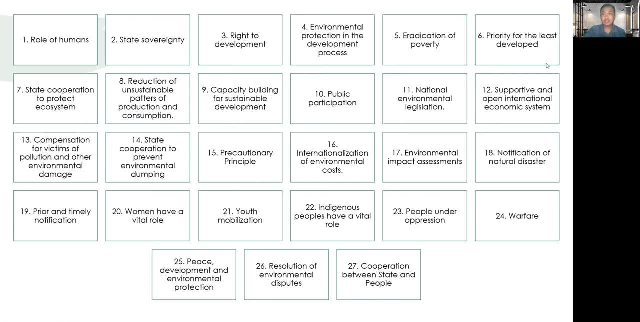 These are the 27 principles stated in the Rio Declaration: One: rule of humans. Two: state sovereignty. Three: right to development. Four: environmental protection in the development process. Five: eradication of poverty. Six: priority for the least developed. Seven: state cooperation to protect ecosystem. Eight: reduction of unsustainable 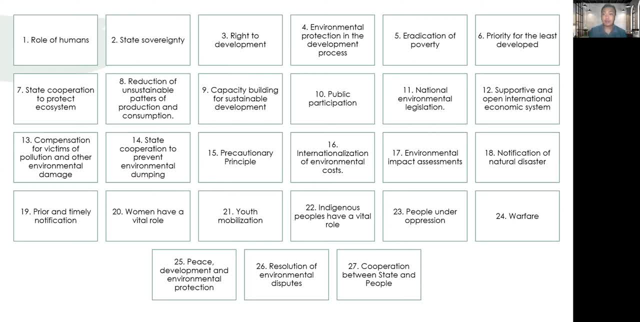 patterns of production and consumption. Nine: capacity building for sustainable development. Ten: public participation. Eleven: national environmental legislation. Twelve: supportive and open international economic system. Thirteen: compensation for victims of pollution and other environmental damage. Fourteen: state cooperation to prevent environmental dumping. Fifteen: precautionary 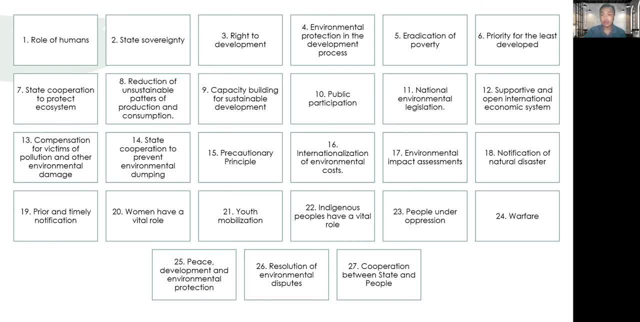 principle. Sixteen: internationalization of environmental costs. Seventeen: environmental impact assessments. Eighteen: notification of natural disaster. Nineteen: prior and timely notification. Twenty: women have a vital role. Twenty-one: youth mobilization. Twenty-two indigenous peoples have a vital role. Twenty-three people under oppression. 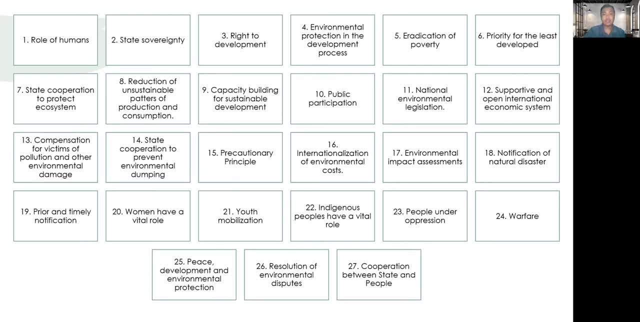 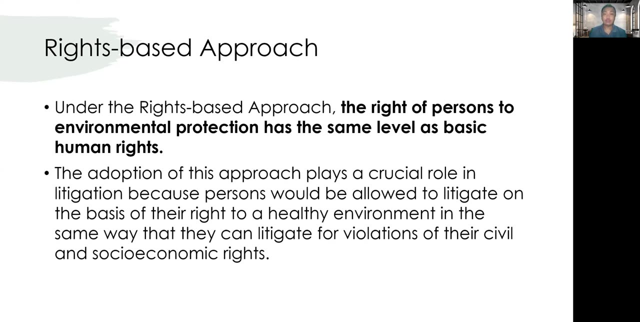 Twenty-four, warfare. Twenty-five, peace, development and environmental protection. Twenty-six, resolution of environmental disputes. And twenty-seven, cooperation between state and people Under the Rights-Based Approach. the right of persons to participate in the development of environmental protection has the same level as basic human rights. The adoption of this 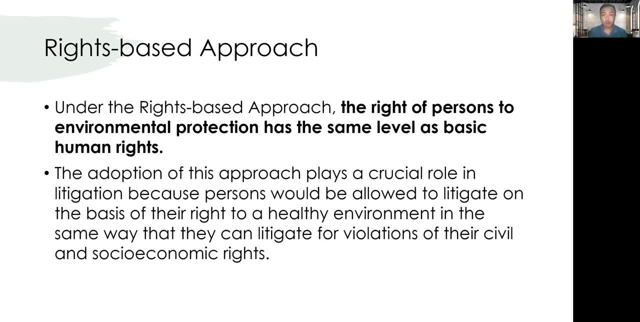 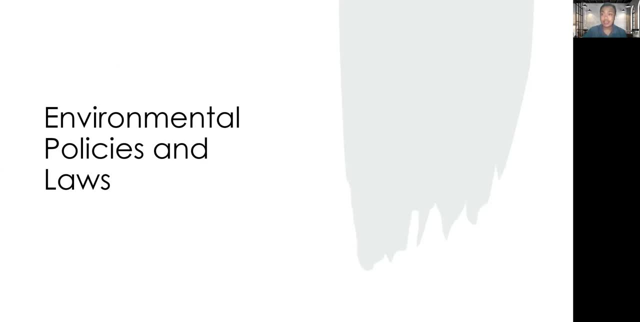 approach plays a crucial role in litigation, because persons would be allowed to litigate on the basis of their right to a healthy environment in the same way that they can litigate for violations of their civil and socioeconomic rights. Let's now discuss the environmental policies and laws. Let's first differentiate policy. 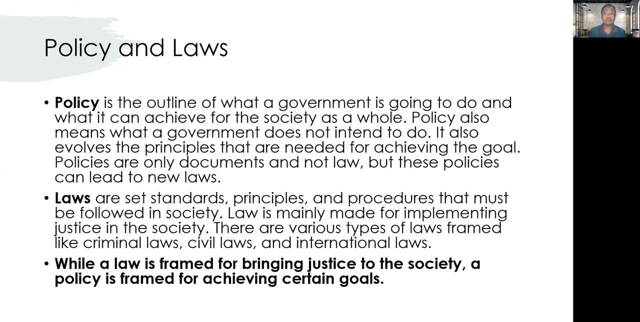 and law. Policy is the outline of what a government is going to do and what it can achieve for the society as a whole. Policy also means what a government does not intend to do. It also involves the principles that are needed for achieving the goal. Policies are only. 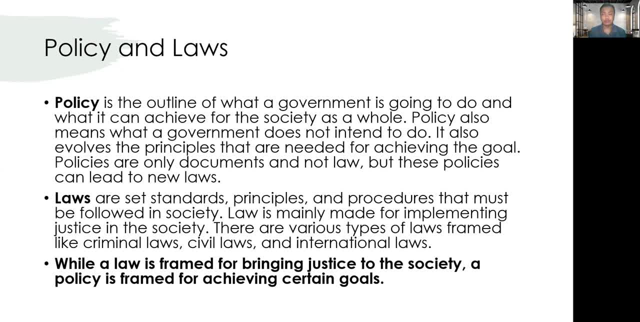 documents and not law, but these policies can lead to new laws. Meanwhile, laws are set standards, principles and procedures that must be followed to ensure that justice is implemented in society. Law is mainly made for implementing justice in the society. There are various types of laws framed, like criminal laws, civil laws and 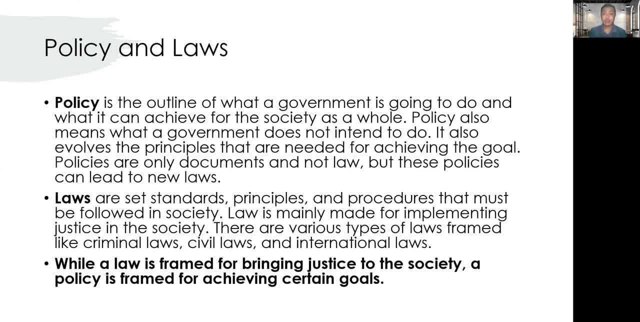 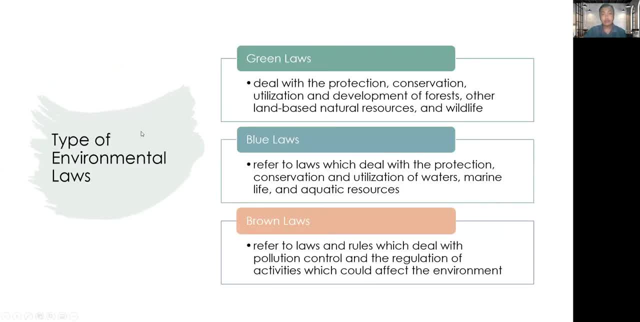 international laws. While a law is framed for bringing justice to society, a policy is framed for achieving certain goals In terms of environmental policies and laws. they are classified according to their nature. 1. Green Laws: Green laws deal with the protection, conservation, utilization and development of forests. other: 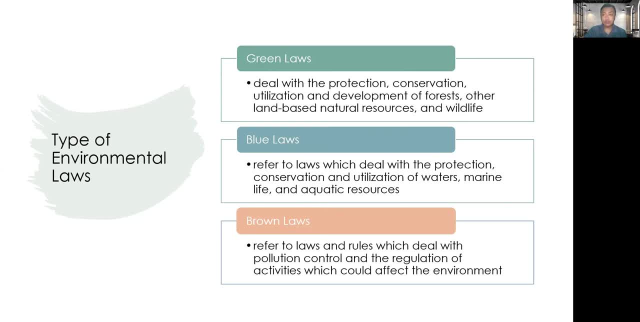 land-based natural resources and wildlife law. 2. Blue Laws: These are laws which deal with the protection, conservation and utilization of waters, marine life and aquatic resources. 3. Brown Laws: These are laws and rules which deal with the pollution, control and the regulation of activities. 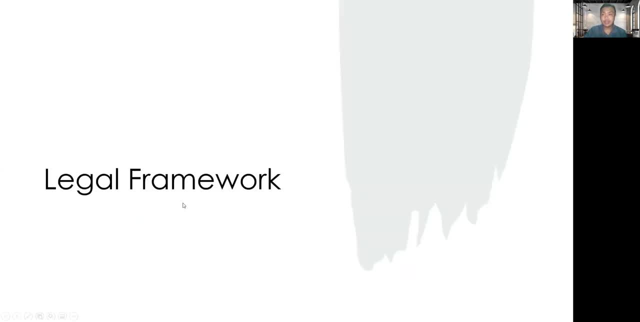 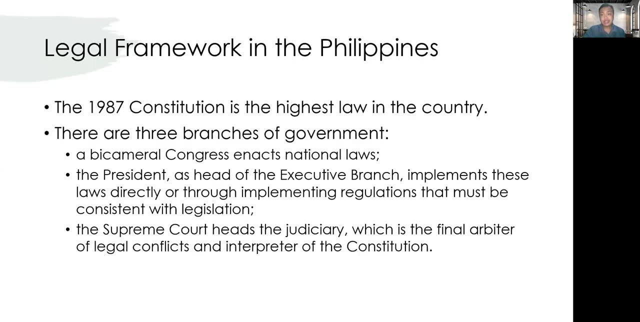 which could affect the environment. This time we'll be talking about the legal framework in the Philippines. The 1987 Constitution is the highest law in the country. We also know that there are three branches of government: 1. The bicameral Congress that enacts the national laws. 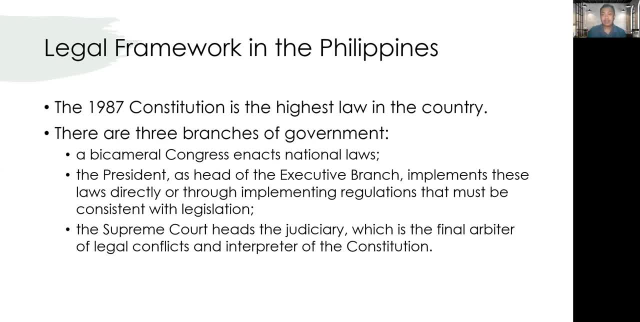 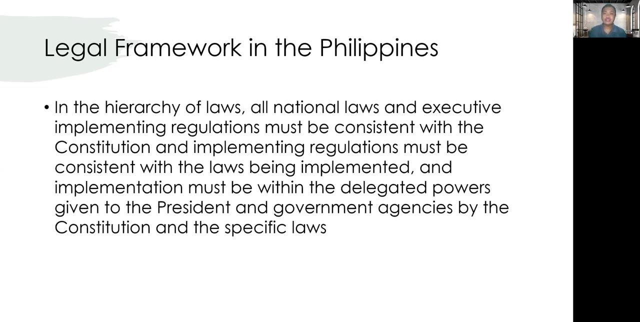 2. The President, as the head of the executive branch that implements these laws directly. 3. The Supreme Court, that heads the judiciary, which is the final arbiter of legal conflicts and interpreter of the Constitution. 4. In the hierarchy of laws, all national laws and executive implementing regulations. 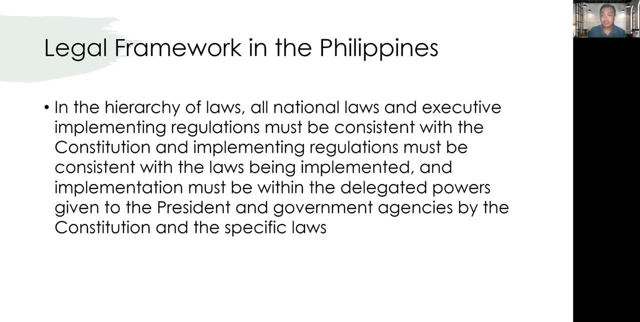 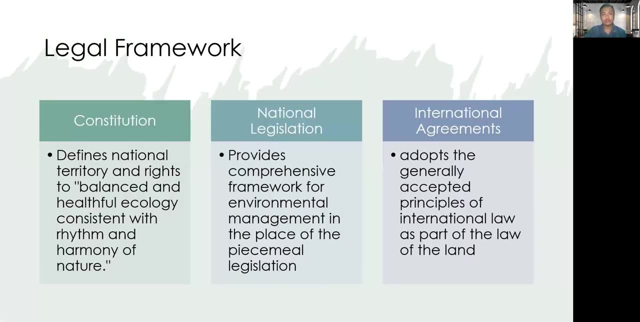 must be consistent with the Constitution and implementing regulations must be consistent with the laws being implemented. 5. The implementation must be within the delegated powers given to the President and government agencies by the Constitution and the specific laws. The legal framework in the country follows these three. 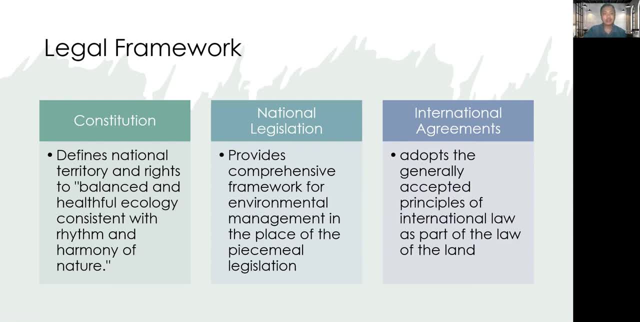 1. The Constitution that defines the national territory and the rights to balanced and healthful ecology, consistent with the rhythm and harmony of nature. 2. The National Legislation that provides the right to the rights of the people and the environment. 3. The Constitution that defines the national territory and the rights to balanced and healthful 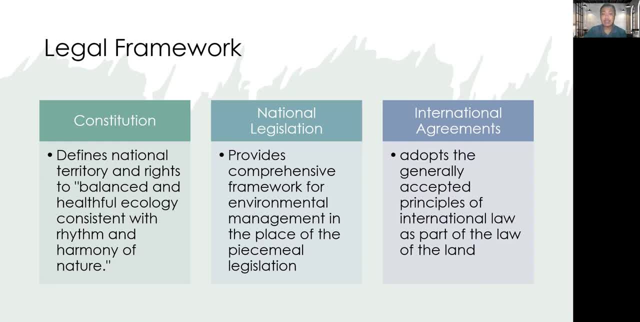 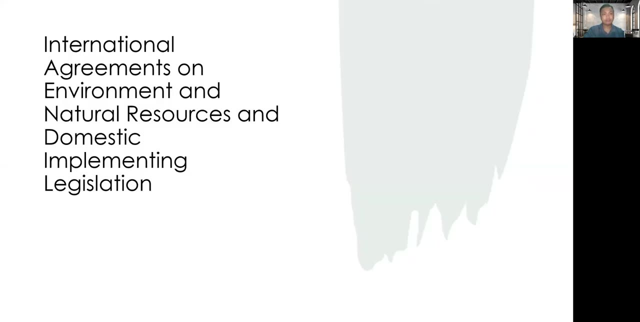 ecology, consistent with the laws with respect to their aquatic life. 4. The 2nd smoking law that does business in the country and recommends Héctoriku, our union chief director. This exploitation of your land is not of your concern. It is cause and effect at hand for you to continue to use any legal means of your home.